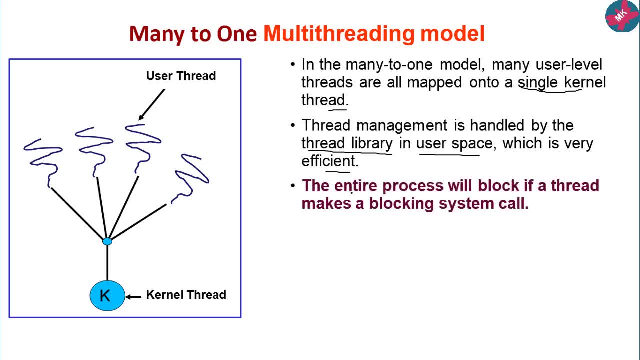 The entire process will block if a thread makes a blocking system call. So, as you can see here, if any one of this user level thread makes the system call, now, if you recall, what do you mean by system call? That is nothing but the interface between the process and the operating system, more. 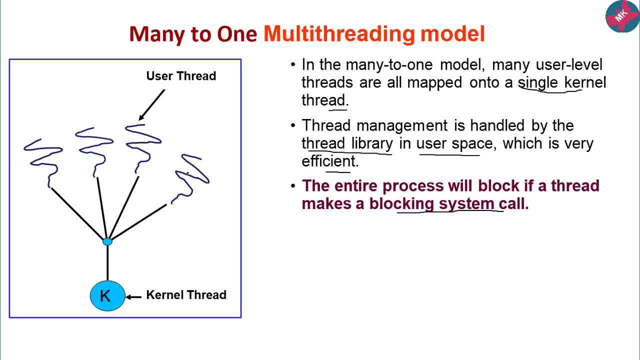 particularly kernel, isn't it? So, say, suppose, if any of this user level thread makes a system call, then what is going to happen is that if the requirement of that user level thread is not fulfilled, then system will be blocked and other user level threads will not be able to access this kernel thread. 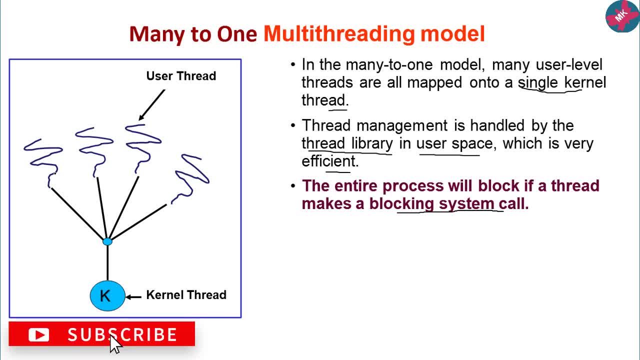 unless and until that system call is resolved. So this is the drawback of this many-to-one multi-threading model. Now, as is seen from the diagram, a single kernel level thread is there and which is responsible for access The kernel at a time. 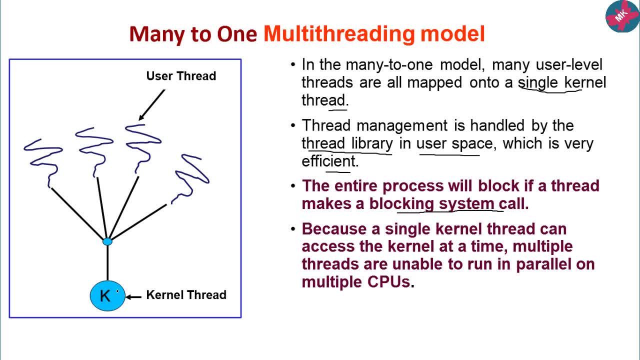 And due to this, multiple threads are unable to run in parallel on multiple CPU, So this system does not permit multi-threading, even if multiple CPUs are available. An example for this many-to-one is green threads for Solaris, and this is particularly used. 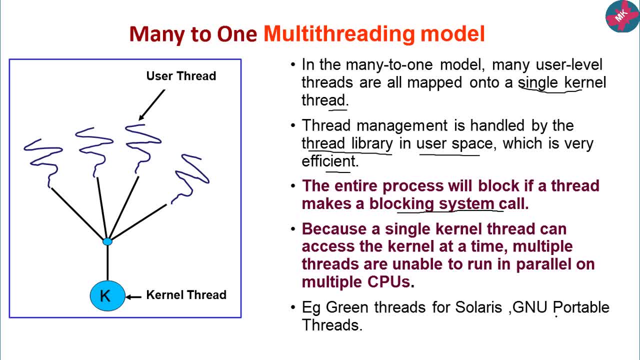 in the GNU portables. So this many-to-one has two drawbacks. First, entire process will block if a thread makes a blocking system call and multi-threading is not possible even if multiple CPUs are there, as there is only one kernel thread. So let us see the next model. 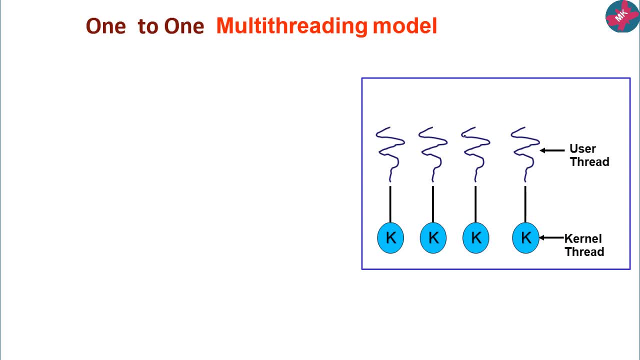 Next model is one-to-one, So here there will be one User Level Thread and for that One User Level Thread there will be one Kernel Level Thread. Here what happens is that here for individual user thread there will be a separate Kernel Thread, and due to this there is more concurrency than the many-to-one model, and this is why. 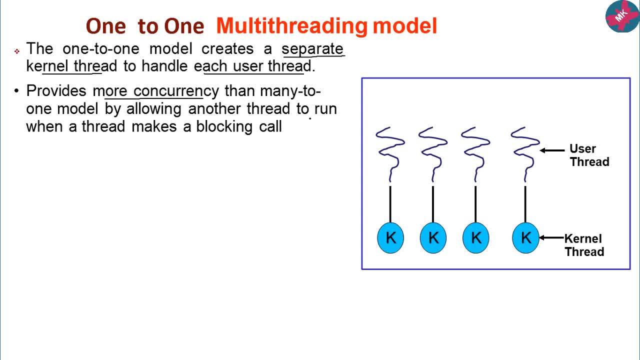 there is one Kernel Level Thread at the end, as each of this user level thread can run independently. so the first drawback that was there- it was there in the many to one- that if suppose one user thread makes a blocking system call, then other user threads will not be affected. 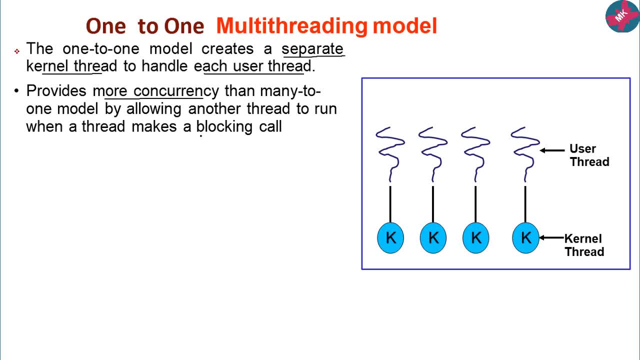 because of that. so the problem of blocking is solved in the one to one multi-threading model and since multiple threads are there, they can run in parallel across multiple CPUs. so these were the two drawbacks in many to one. so these are resolved in the one to one multi threading model. but there are some. 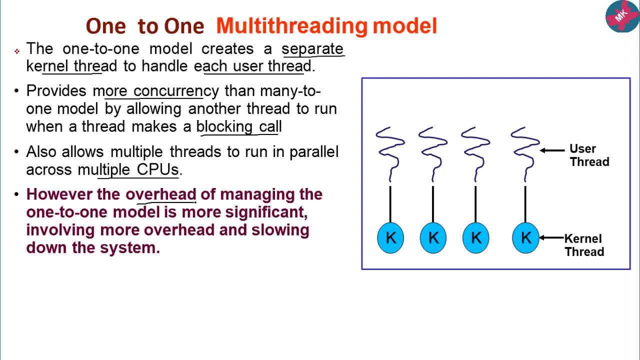 drawbacks. the first drawback is that there is a significant overhead, as, for every user level thread, have to create the individual kernel level thread and due to this, the system eventually slows down and due to this, what happens is that any systems place a limit on how many user level threads can be created, since creation of kernel level threads is quite a significant 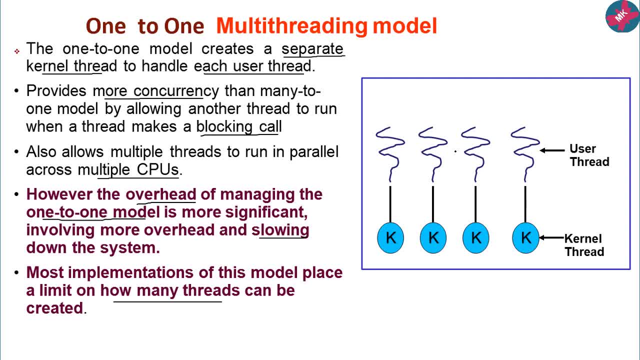 the system may limit the number of user level threads that can be created in a system. So these are the two drawbacks of this 1 to 1 multi-threading model. Now we have seen many to one example, so similarly here the example of 1 to 1 is Linux and Windows. 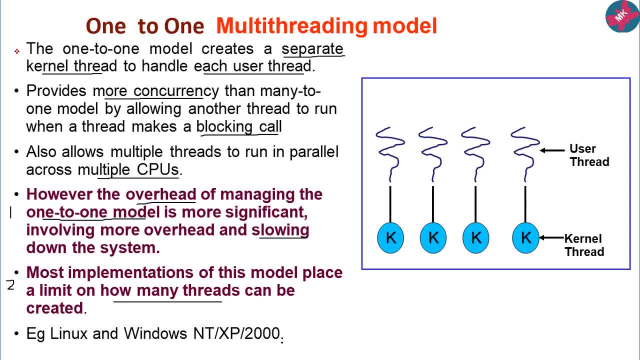 NT or any other version from NT onwards XP 2000.. Now we have seen many to one example, So similarly here the example of 1 to 1 is Linux and Windows NT or any other version from NT onwards XP 2000.. We have seen both many to one and 1 to 1 multi-threading model. 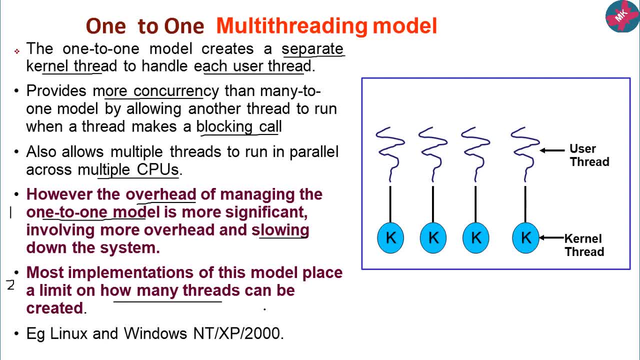 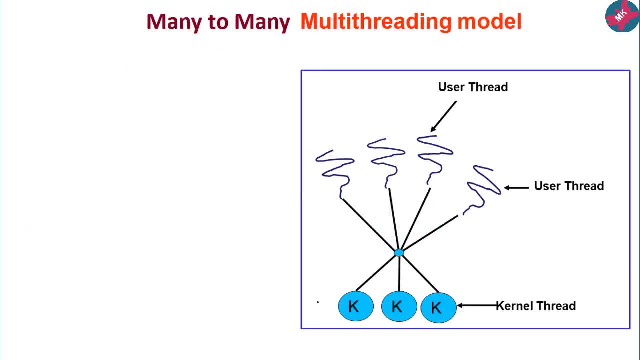 So let us see how the drawbacks of these two models can be overcome. in the third model that is many to many. So here in this diagram you can see that there are many user level threads and there are many kernel level threads. So here there are in this example four user level threads and these are mapped to three. 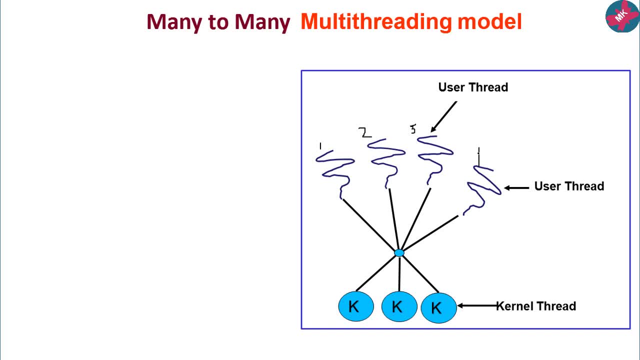 kernel level threads. So here what happens is that many user level threads are multiplexed to smaller or equal number of kernel threads, Like in this example: four user level threads are mapped to three kernel level threads, and this number of kernel threads may be specific to a particular kernel. 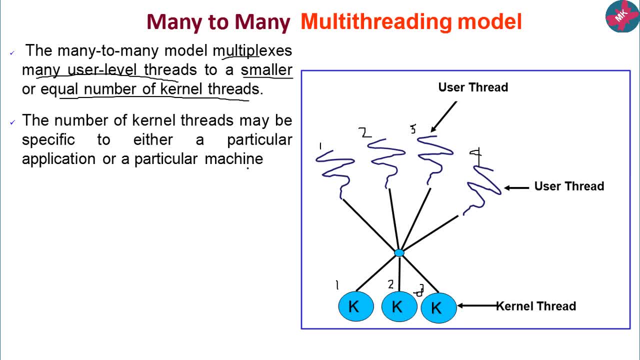 A particular application or a particular machine. and due to this, what was, what was the drawback in the earlier system? that there was limitation on how many user level threads that could be created. So that is removed in this system. So in this system, the developers can create as many users as they consider it necessary. 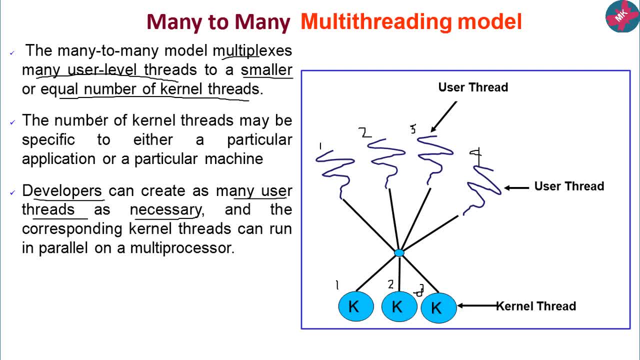 because you don't have to create individual kernel threads for them and this corresponding thread can run in parallel on multiprocessor. So here in this example, three kernel level threads are there, so they can run in parallel on different processors in this particular model. Then the second drawback of the earlier system was the problem of blocking. 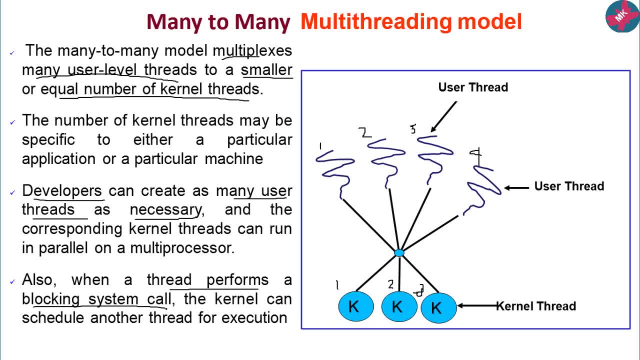 So here, what happens is that, say suppose, if some of the thread initiate blocking, then the kernel can schedule another thread for execution. So whatever was the drawback of the earlier two system, that is, blocking and the limitation on the user threads- that all is solved in this many to many multi-threading model.